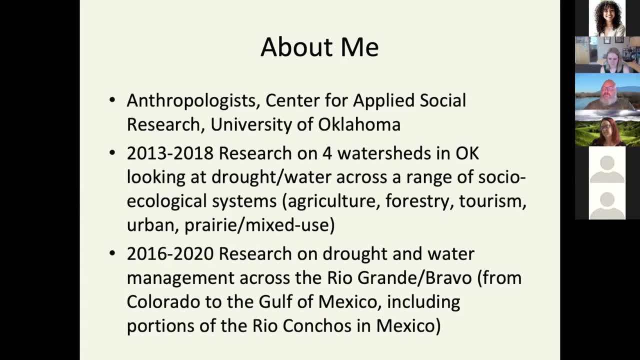 about a five-year project, a lot of intensive in situ research looking at drought and water across a range of socioecological systems in Oklahoma, So very focused on sort of the state but also kind of the watershed level And then also generously funded research through the South Central Climate Adaptation Science Center. 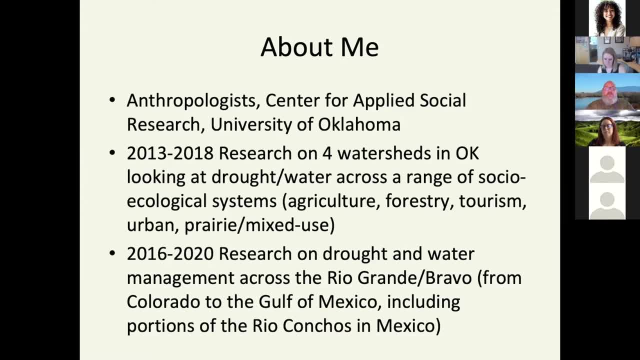 working on the Rio Grande and Rio Bravo, looking at drought and water management. That goes literally from the headwaters all the way to the Gulf of Mexico, includes portions of the Rio Conchas, So today's talk is specifically going to be about the climate adaptation research. 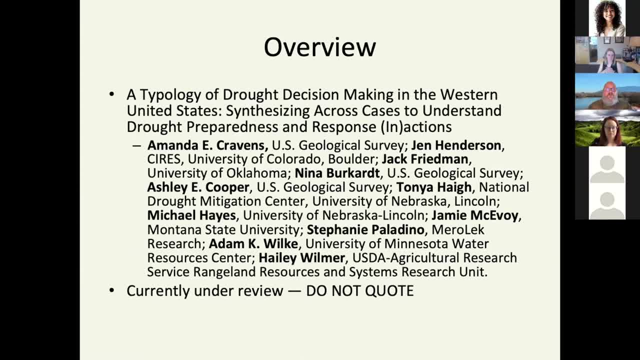 We focused on sort of talking through some of the elements in a paper that we have currently under review. One thing I like about this paper it's about the typology of drought decision making in the Western United States, So really trying to understand drought preparedness. 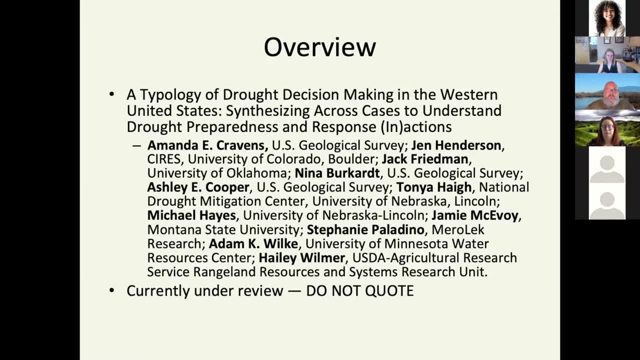 and responsiveness from the standpoint of what is actually being done rather than what should be done. So we start with kind of a description of what's happening rather than you know, starting from kind of an idealized form With a lot of partners, if you take. 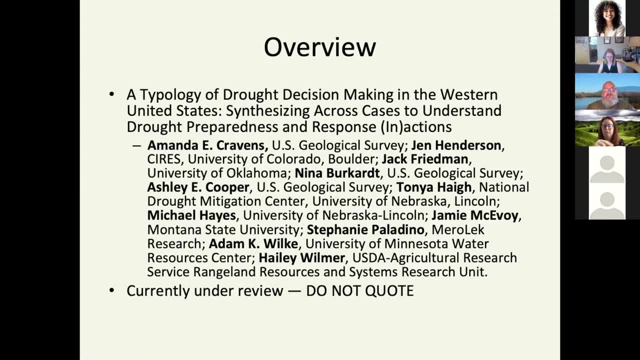 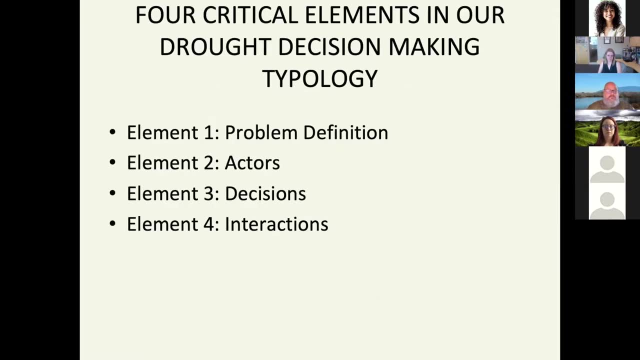 a look at this list, we have everybody from Fed, folks from USGS, USDA to sort of your more standard issue, academic types and even some private folks in here. So, specifically, I'm going to focus today on how our understanding of different typologies of drought decision-making. 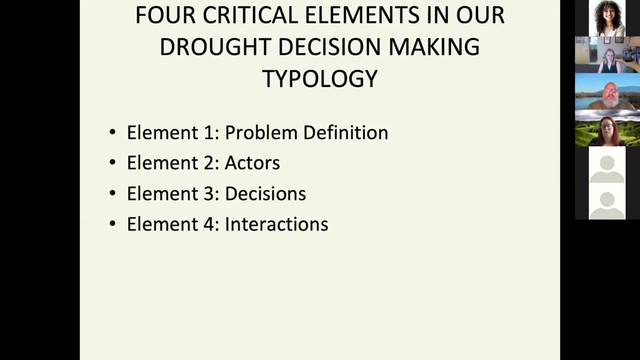 might prove helpful for resource managers who are dealing with the evolving landscape of climate change-related drought challenges. So I'm going to break this up into the four elements that we've kind of identified, each of which has a number of dimensions, So it can get complicated, but I think if most folks on this call are resource managers, this is 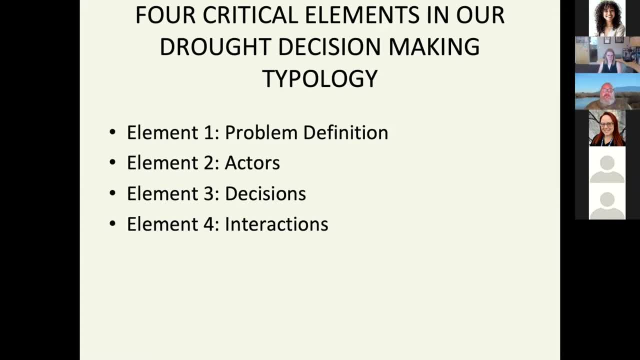 a fairly easy story to follow. So element one focuses on how drought is defined in practice. In the first place, what you'll see is that I don't care about the book definitions of drought at this stage. What I really want to look at is what resource managers actually 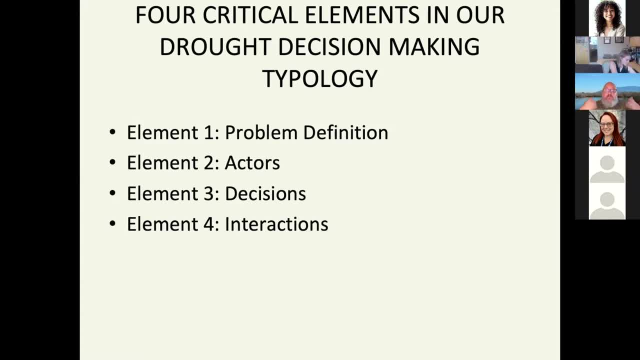 do and to use that to figure out a typology. Element two actually looks at the question of who those actors are, who make who we can count in the sort of universe of drought decision-makers. Element three looks at the kinds of drought. 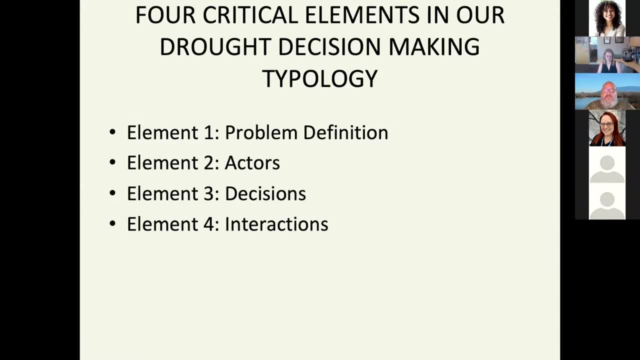 decisions that are usually made by drought managers and why this matters in a climate change impact-impacted world. And finally, element four looks at how, why and when interactions between drought decision-makers impact. So the interactions is the key thing here. impact. 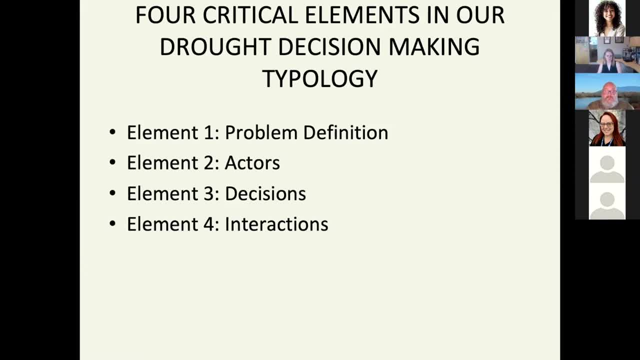 the success of drought adaptation strategies, So we'll do a few interactive polls. in between each of these brief discussions, though- And I think I'm having a lot of fun- I'm hoping that folks will add into the chat a few questions about why in the world these 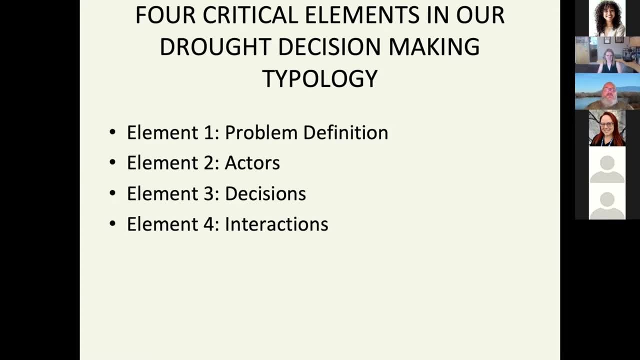 particular questions were included in this poll because I'm trying to not only get information but actually prompt you to think in a certain way. So, Emma, if you can, could you launch poll number one? We've run these polls before and this one in particular takes about two. 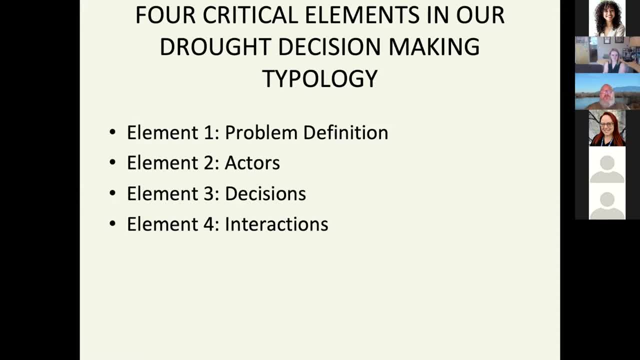 and a half minutes usually. You'll see there's a lot of repetition in the questions And the way that you answer them, So please dive right in. Thank you, Thank you. So I'd like to close this in about 20 seconds, 30 seconds if possible. 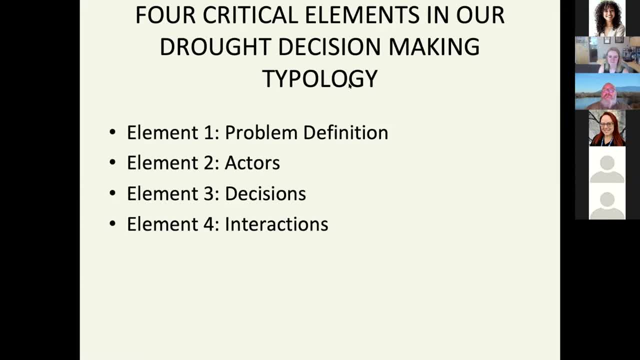 All right, so I'm going to close this in about 20 seconds, 30 seconds if possible. I'll close this in ten seconds, All right, so So I'll close this in 10 seconds. All right, So I'll close this in 10 seconds. 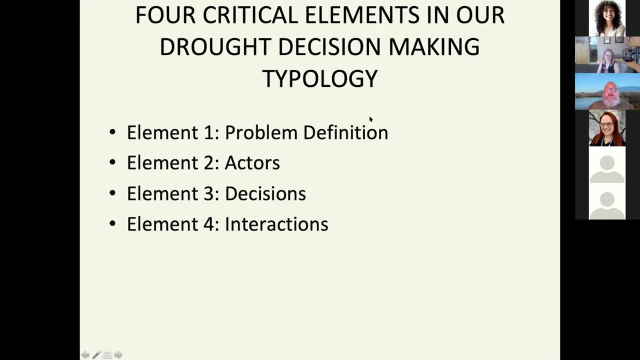 All right. So if you could please start the poll again, please mean, I'll do a quick share of the results. It's. you know this isn't a great way to show these polls. I'm not sure, Emma, how many polls have been done so far, but I apologize for the lack of 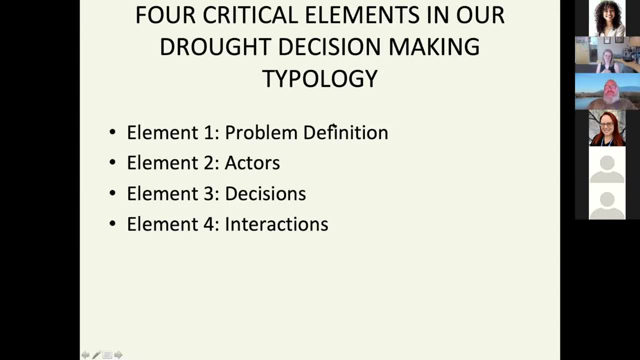 ideal graphics here, But you know, this is kind of what Zoom gives you. So obviously it's interesting to me to see the sort of difference between folks who are going to give sort of explanations that are really heavily focused on drought limitations based on physical things. 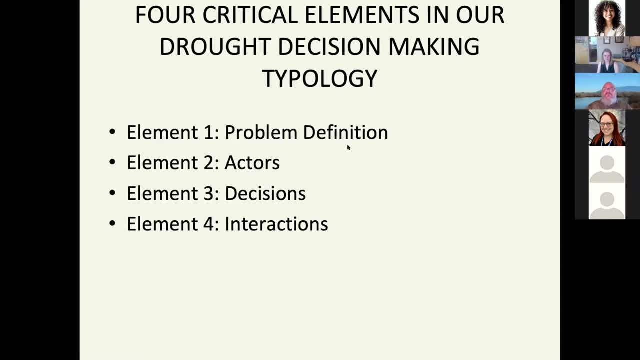 which we can see are sort of floating around, the sort of that most people have. given it that I'm intrigued by the person who says not limited at all, because I think that's really interesting. You can also see, obviously, a very high role that's being played by politics and policy. 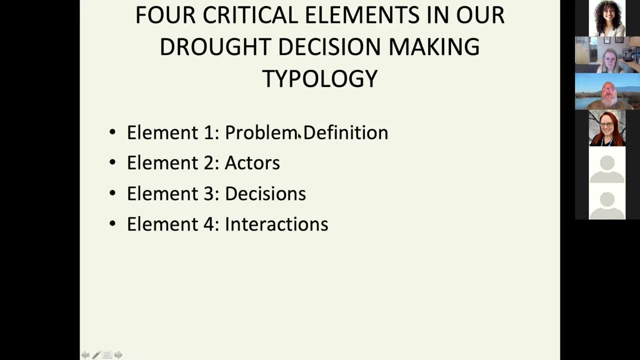 and I like this sort of moderately driven by engineering and new technologies. Depending upon the audience that you're talking to, that can be extremely high, extremely low, and I think it's interesting that in our group that it's kind of in that moderate range. This issue of changing. 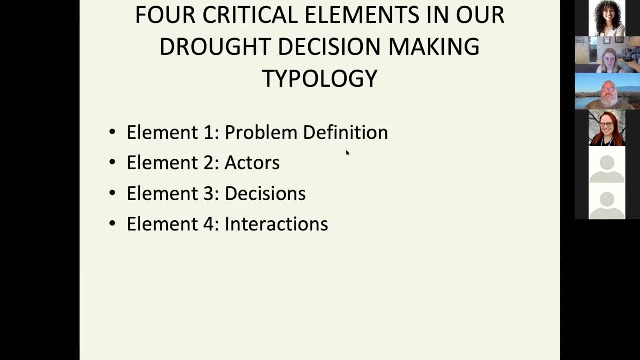 human behavior. I think it's good that sort of fits into my wheelhouse. But again what we have is a lot of balance across the board. all of these things, Almost everything, is in the moderately to significantly driven category. There are very few cases here where one says that it's entirely driven by one or the other. 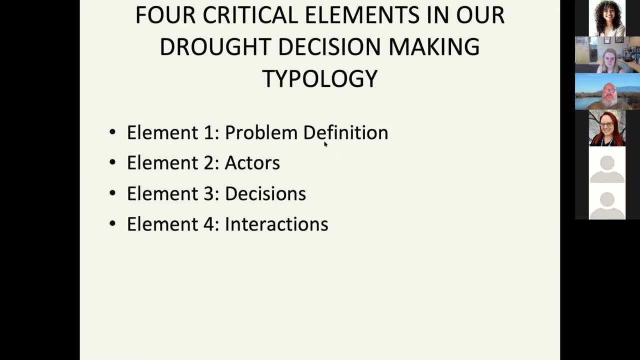 So we have one person who said that it was entirely driven by natural and physical processes and one person who says it's entirely driven by human behavior and perception of problems and drought. But beyond that, you see that this complex mix of factors and everything is kind of 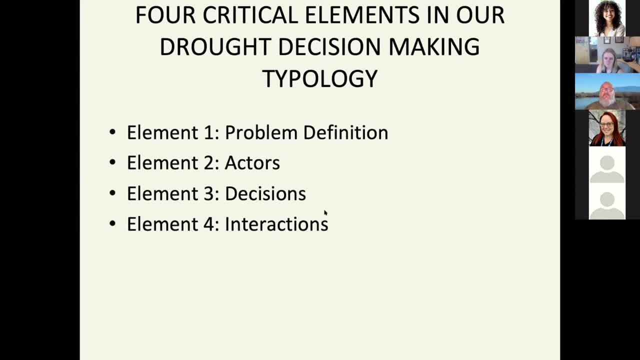 moderately or significantly for most people. I think tells us the sort of complexity of some of these challenges that we're facing, that they're not just a physical problem, It's not just a problem with people or politics or the economy, but it's this combination of factors. All right. 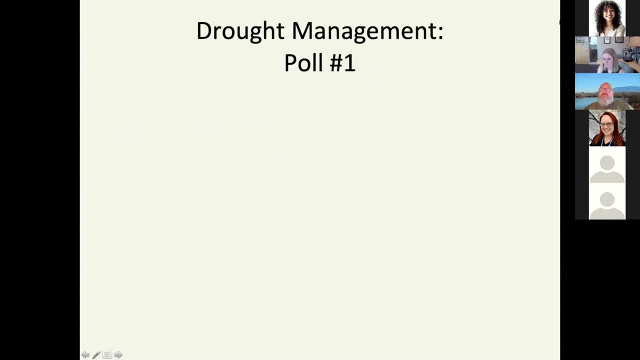 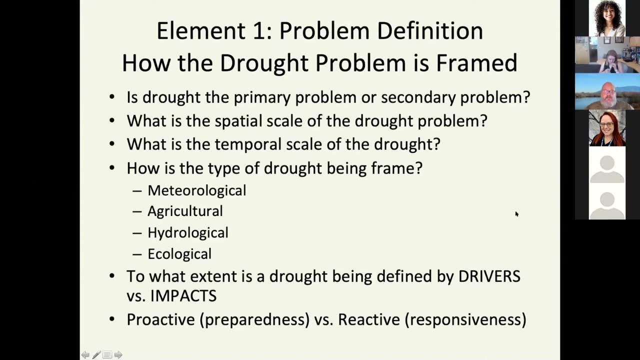 so let me move back to my slides and talk a little bit about the four elements that we have in our typology. So element one focuses on how drought is framed as a problem and why that matters in understanding adaptation to climate change influenced drought. Our research brought together a number of different 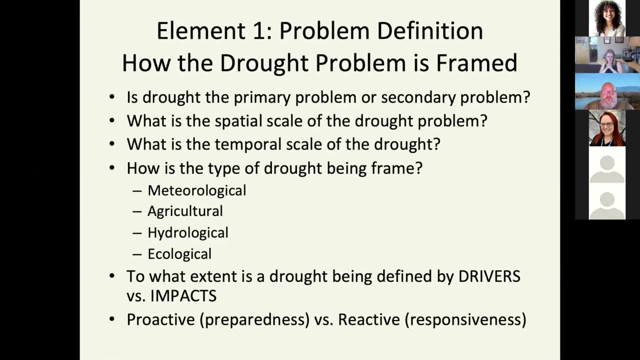 elements that play into the definition of drought problem. So first we saw that some drought decisions focused on drought as a primary problem and other decisions focused on drought as a primary problem. So we saw that some drought decisions focused on drought as a primary problem and other 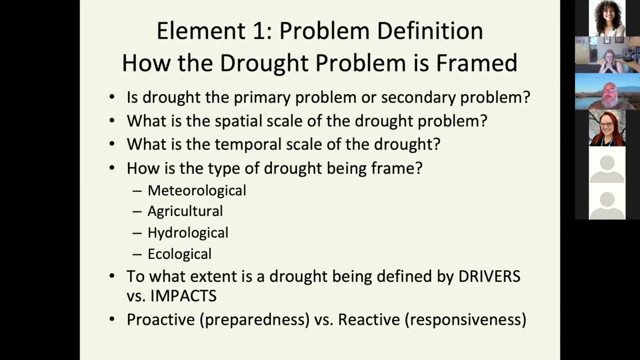 decisions focused on drought as a secondary problem. That might not be really obvious what I mean there, but I'll explain it in the next slide. Hopefully it'll be a little clearer. On the other hand, I suspect that these next two elements are very clear, that some you know that, how one defines drought as a spatial 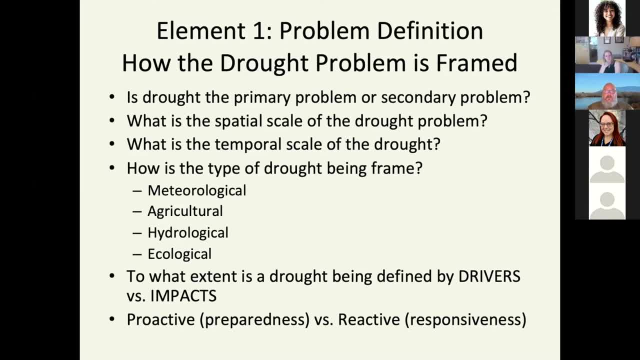 problem versus a temporal, or a temporal problem will be much more obvious to many of you. In some cases we have actors, so drought managers, who are very clear about the type of drought, And then we also have a set of risks, so that's a big one. So just to sort of explain more on the 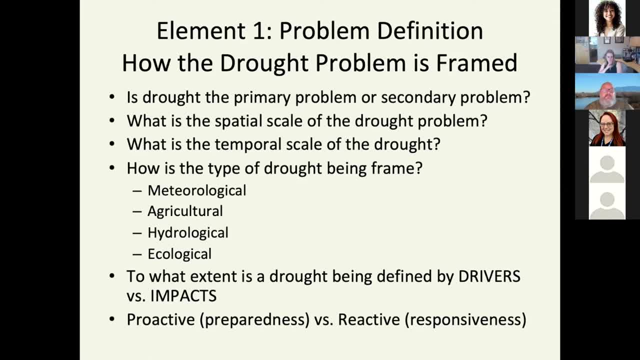 different ways that we're looking at it. So we looked at how many people are thinking about drought, how many people think about how they're thinking about the weather, how many people are thinking about Requirements to be proactive- So focusing on preparedness versus reactive- all of which seem like very different elements, and they are very different elements. 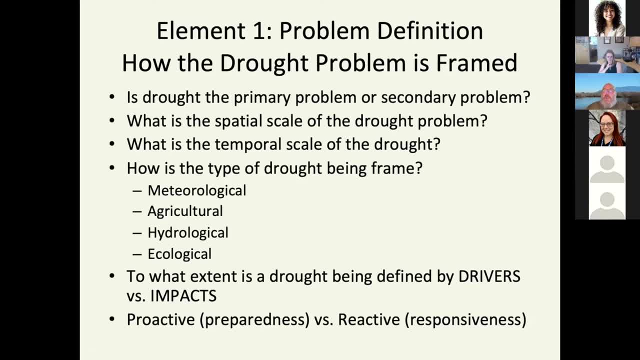 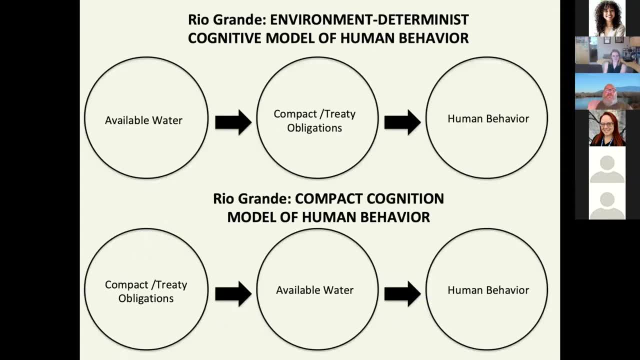 There's no way I can talk about all of these. We'll be here for hours, So I'm just gonna focus on a couple that I think are maybe a little bit. a Little bit either unclear or very illustrative. So the one that I think is the more unclear one. 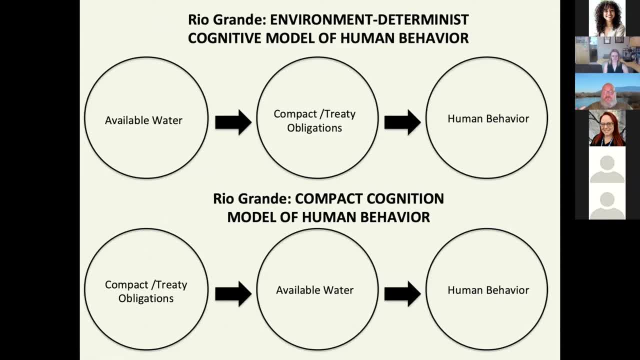 Is this issue of primary versus secondary? and yet I think it's really important. I'm going to use an example from our research in the Rio Grande. In different parts of the Rio Grande, resource managers consider drought in different ways. for some, Drought itself is the driver, meaning that they assume that the environment 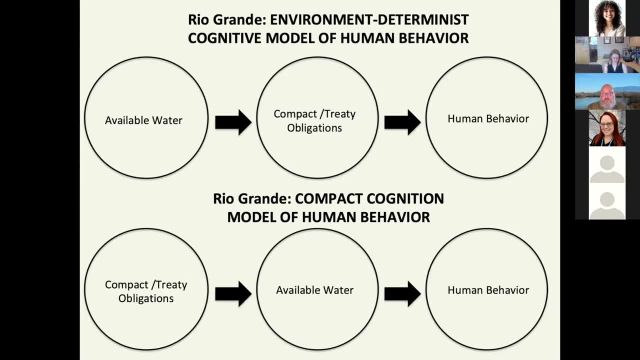 Determines the actions that they can take. too little water leads to requirements to implement various portions of water treaties and agreements. You can think of this as kind of algorithm thinking: We're lacking water, therefore we immediately click this switch and, And, and in turn, this forces humans to take specific actions. 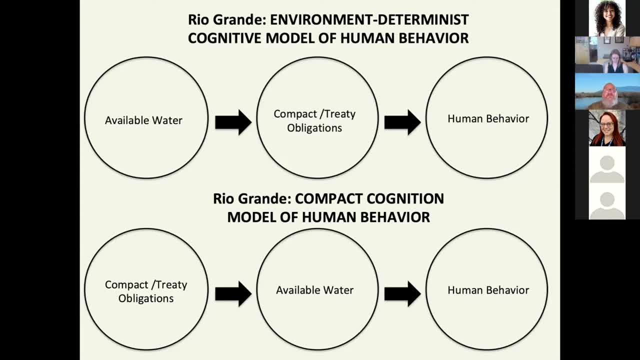 So this is what I would term the environment determinist model of behavior. In other portions, though, of the Rio Grande, managers see That it was specific human actions in the first place, and The way that water is consumed, the impact of reservoirs, the role of agriculture, etc. 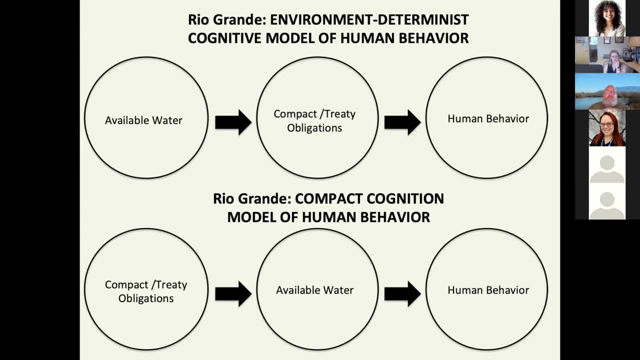 That has created the drought conditions. in other words, that, yes, you might have limited precipitation during a particular year, But that that would not be cascading into catastrophic agricultural Or or other ways of thinking about agricultural or hydrological Drought if we didn't have this, this sort of human man in engineering of the landscape, in a 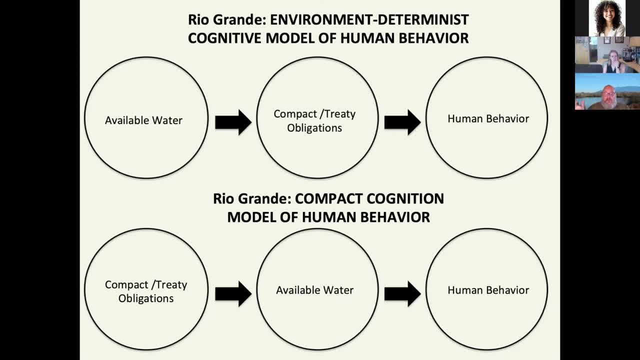 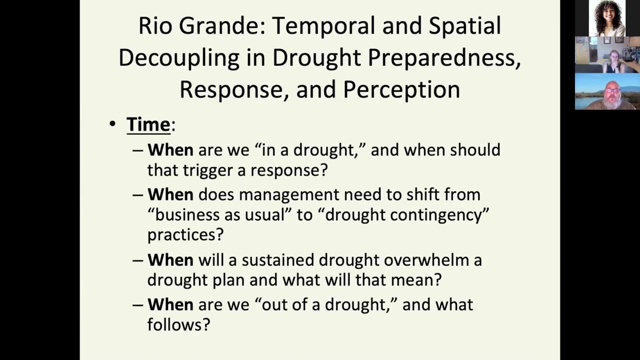 particular way. so each of these ways of framing the problem of drought ends up defining the decisions that can be made, and this is what I mean by drought as primary versus drought as secondary- perhaps probably a more, a more obvious way of thinking about the way that we. 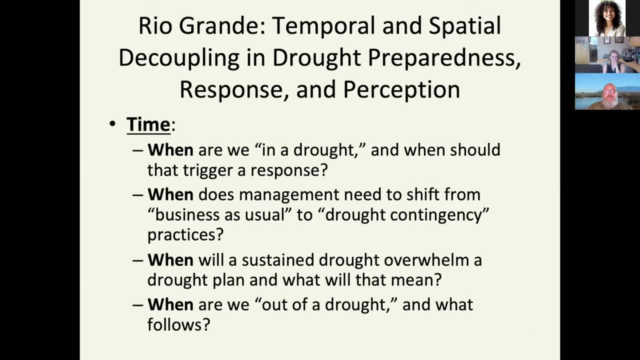 define drought is sort of from a temporal standpoint. so time obviously has a big role to play here, because it defines when we are in a drought and when should that drought trigger a response. when management needs to shift from business as usual to drought contingency practices, when will a 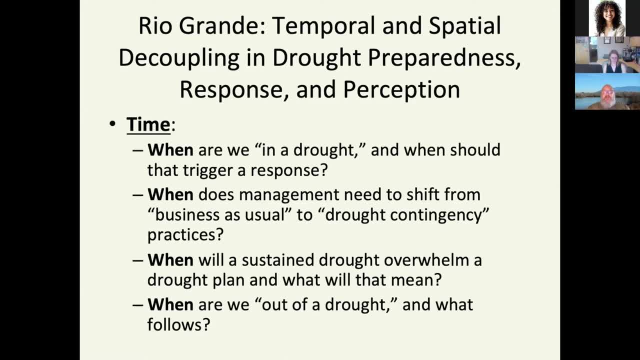 sustained drought, overwhelm, a drought plan, and what will that mean and when are we out of a drought and what follows each of these sort of, each of these questions, each of these sort of dimensions end up defining kind of how a drought is defined in the first place. 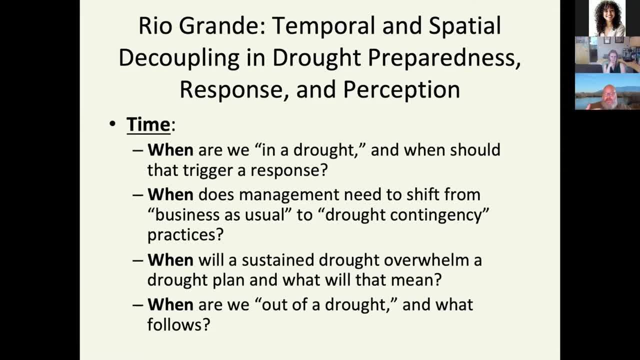 and again we recorded all of these different ways of thinking about this, from the drought managers and resource managers who were included in all of our studies, and all of these different places in the West. so again, I'm just reporting on the Rio Grande a portion, but the co-authors on the study of 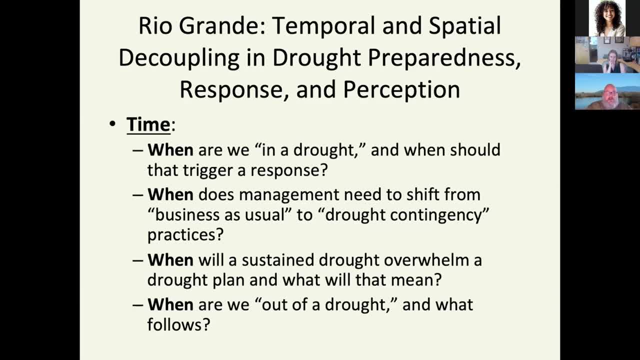 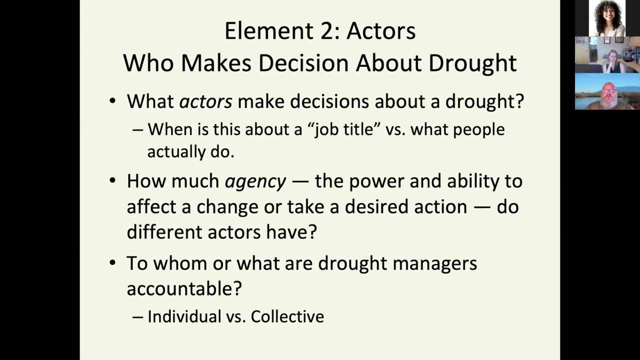 we're doing work all throughout the West. element two in our typology simply looks at who counts as a drought decision-maker. so we very quickly realized in our study that falling back on simple job titles or job descriptions was inadequate if we wanted to understand a typology of. 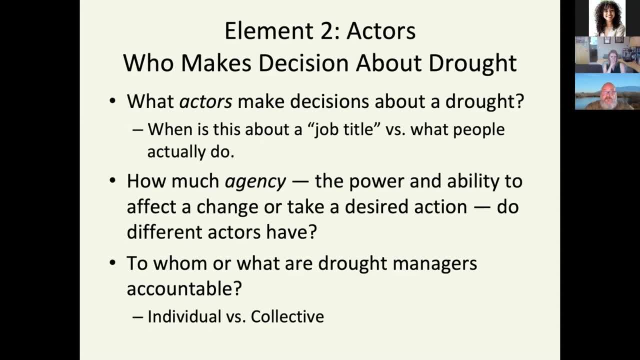 drought decision-making. thus, while most formal drought managers were also types of resource managers, we quickly realized that we could not exclude, for instance, farmers and ranchers, whose decisions before, during and after a drought could often mean the difference between drought and not drought. at the same time, we were acutely aware that some people who manage resources 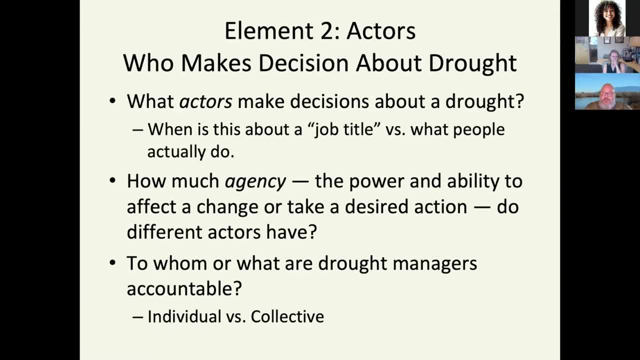 actually don't have much agency, meaning the power and ability to affect, to change or take a desired action, so they might not be included in our, in our typology, um. this is the kind of lever puller um idea that somebody sort of gets a, gets an order, and their job actually is simply, you know, figuratively or literally, pull a lever. 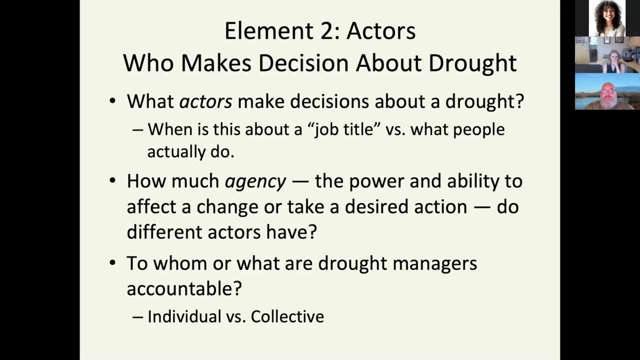 they're very important for the flow of water, for decisions that are made, but they might actually not be making those decisions. um, finally, we also considered whether or not an actor was primarily tasked with making drought decisions for themselves, so that would be sort of household, their households, farm, ranch, business, etc. or whether they were responsible for acting in. 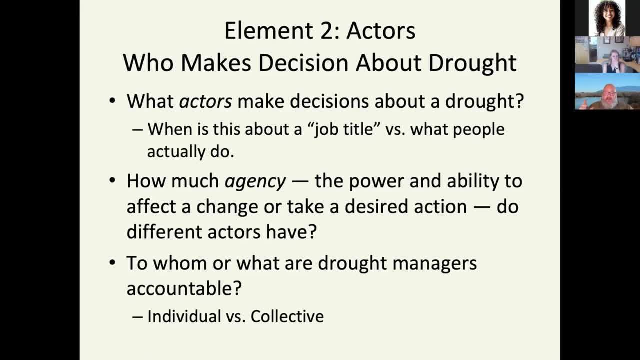 the collective best interest. so each of these dimensions um also kind of shaped the type of drought adaptation planning that we were able to observe in our research. and all of this leads me away from my rambling and lecturing um and hopefully moves us into something in the future that we're going to be able to use in our research. and all of this leads me away from my rambling and lecturing um and hopefully moves us into something 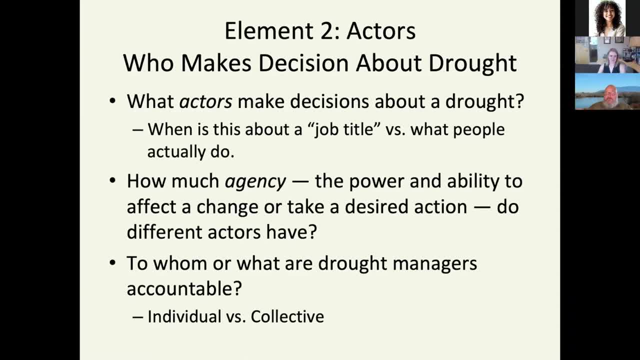 again a little more interactive. um, so at this point, um, can, emma, can you launch poll number two, and hopefully you'll see the thematic similarity here again. this poll usually takes about two and a half minutes. we'll see whether or not we sort of stick to that. but go ahead, jump on in and you'll. 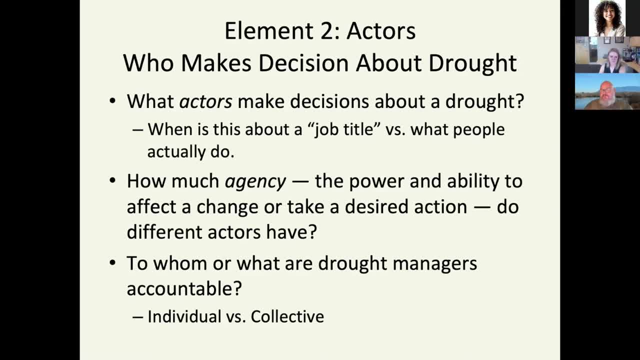 see there's a lot of opt-out uh answers for those of you who are not resource managers at all these users today. so i'm going to go ahead and press that and we will have them in our chat. so if i'll just wrap this up with a few words, 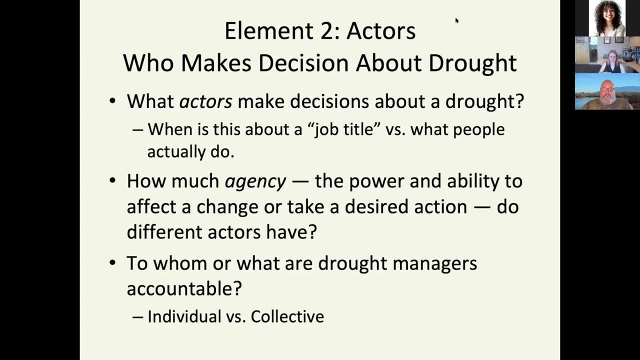 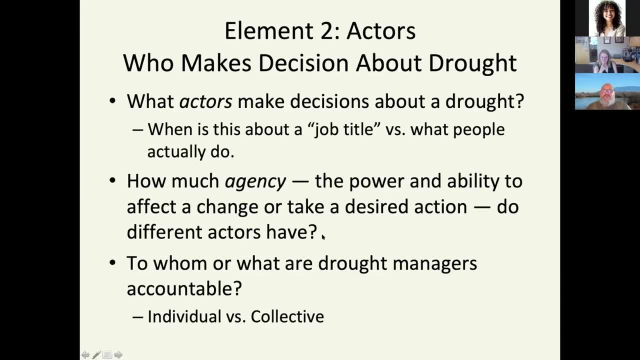 I hate cutting people off. So this is one of the sort of key things that we found in our research afterwards, As I was sort of driving home with this sort of discussion in the first place- is that, if you just focus on people whose formal roles is something. 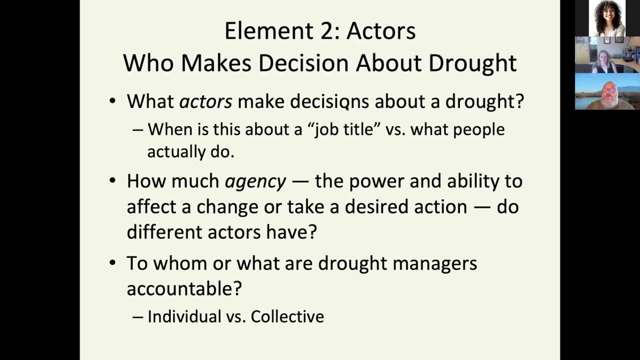 having to do with drought. you end up with very few people. Instead, drought falls under many other people's category, you know sort of a broader umbrella. So we have a lot of people who don't think at all that their, that their job is to manage for drought in this community. 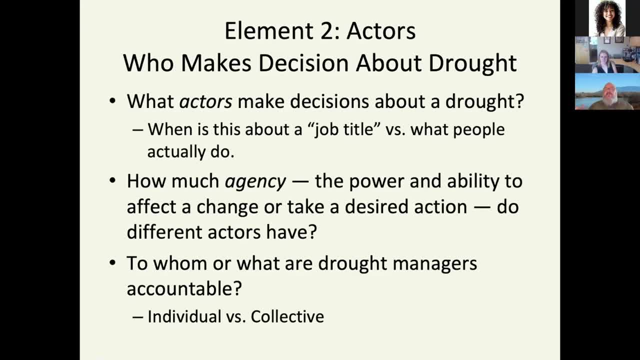 Again, I'm not sure who's on today. I got a list in the first place of some people are academics. We've got a lot of other kinds of resource managers And yet, as you sort of work your way through, people are aware enough of the fact that their organization broadly might be. 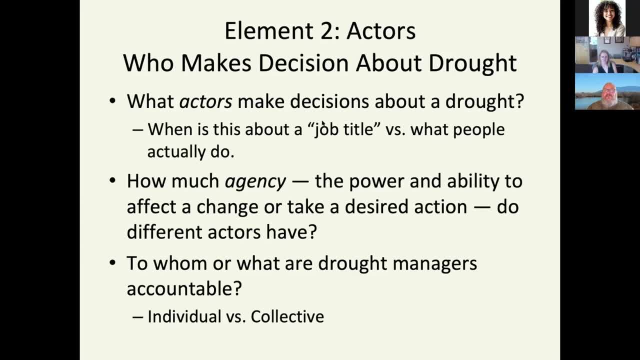 managing for drought. I think across the board it looks like only about about a third of the folks who answered things actually are in an organization that does not manage for drought, which means that everybody else they're sort of becoming very aware. You can see this nice split between regions sort of where people are managing 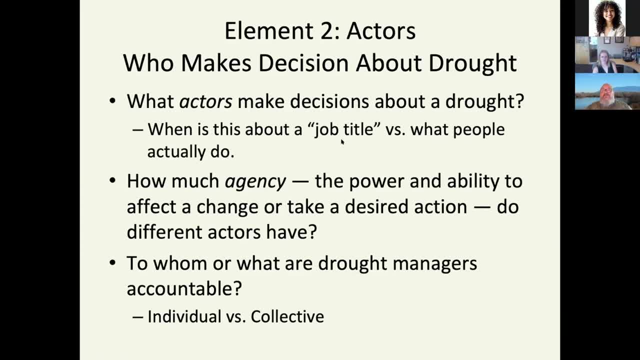 as well as the different kinds of types of drought that they're managing for. I would be really interested to see what ecological drought actually means for other folks. If anybody wants to throw anything into the comments about ecological drought, I'd be really happy to do that. 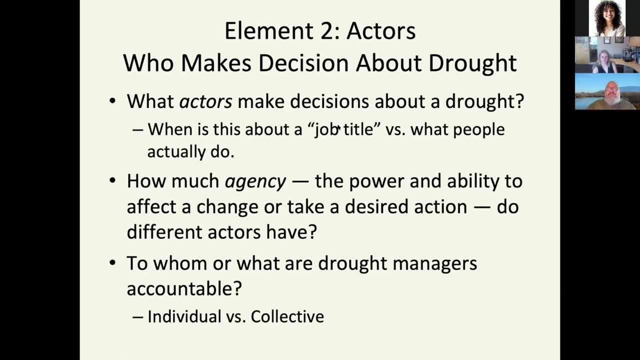 And I think we've got time for one last question. here We're going to go to the next slide, which is well, I know that the word drought means blank for our organization. I know this is kind of very rapid pace here. 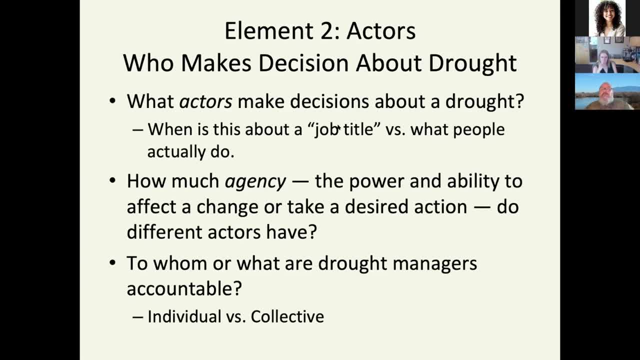 so you might not have time to do it, but I would love to hear what you're thinking in terms of those terms and and how how it kind of plays itself out. Also, I think it's incredibly telling that nobody thinks that their organization is. 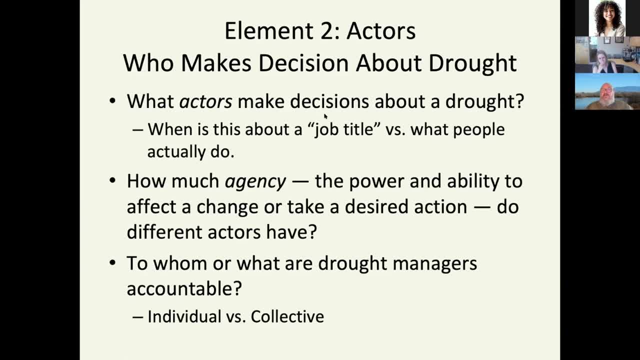 managing for the drivers of drought. Everybody is mostly managing for very telling, and it's it's also interesting to me the sort of balance between preparedness and response, although it looks like I might have cut this off a little early. I'm sorry if I did. I'm just moving by, we're gonna run. 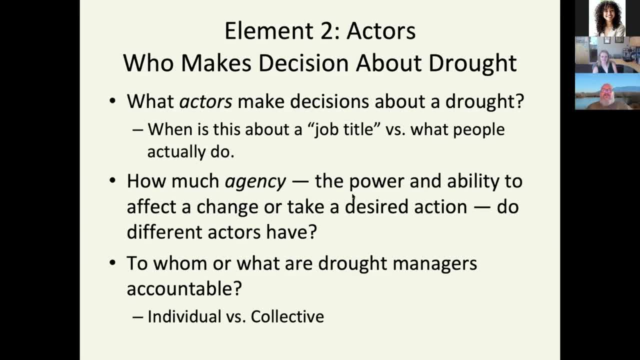 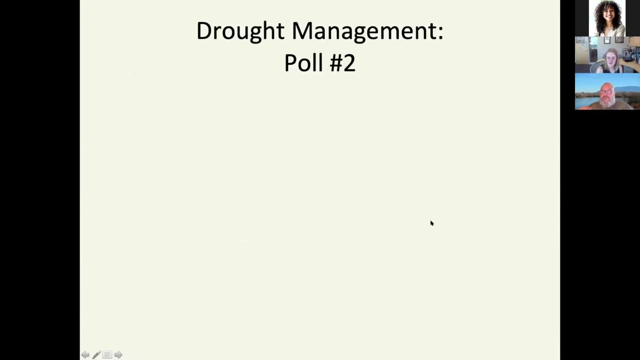 out of time otherwise, because there aren't as many responses for this last question, so I'm gonna stop sharing. I want to move on so I don't run out of time here. it does like look like you. you have someone. Chris says ecological drought to him means threats to at-risk species and natural communities. yeah, and. 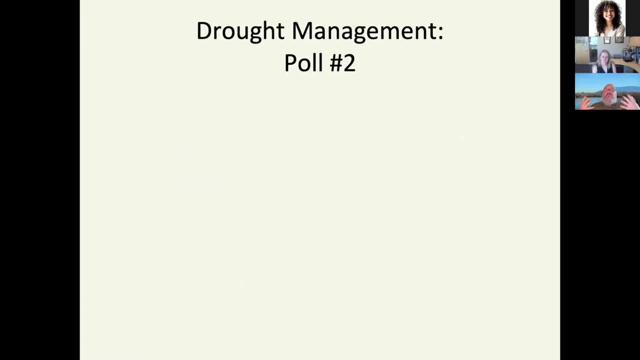 that's really the sort of way to think through it, especially if you look at published work by at least some of the co-authors that are on the current paper that we have that this is under review, who were involved with the development of this project, and I think it's really important. 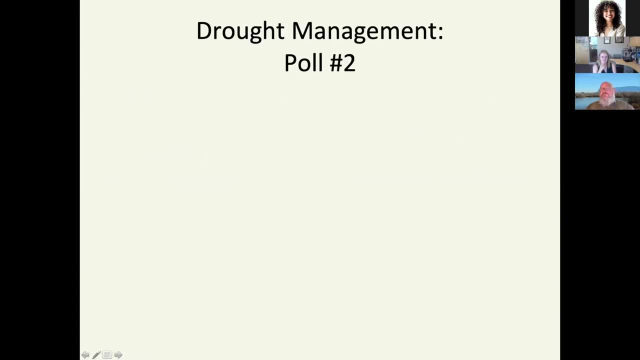 with kind of this broad effort by a bunch of USGS people and other folks to try and define what eco drought would mean, how it's different than related to, but different than the three other traditional ways of thinking about drought. so it's nice to hear that that's the way that folks are thinking about it. 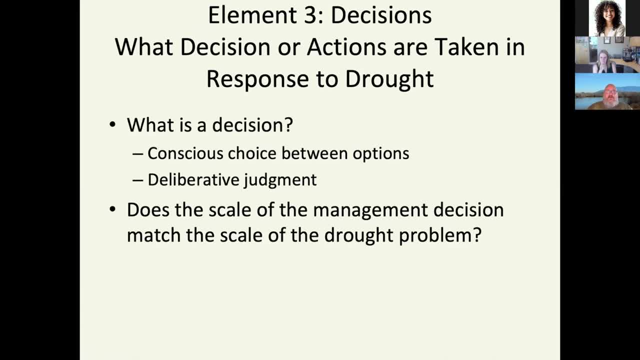 so let me move on to the third element in our typology. so, getting back to this typology, element three looks at the different types of decisions that are made regarding adaptation to, in response to, drought, and so, first and foremost, what we had to figure out was: what was a decision? this? 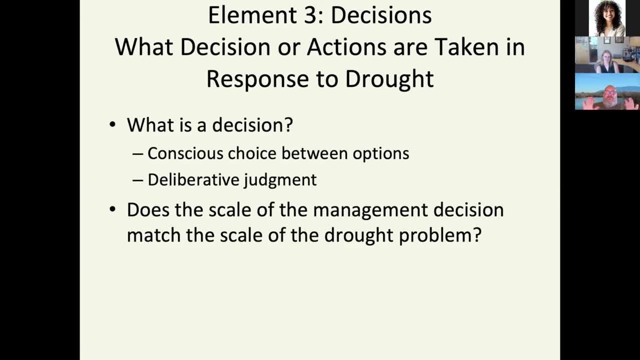 is important for us because, in order to be a decision, one has to- can't be able to consciously- make a choice between multiple options, and that there must be some level of judgment here and again. what we're trying to distinguish between the two is that we need to make a distinction between those who do. 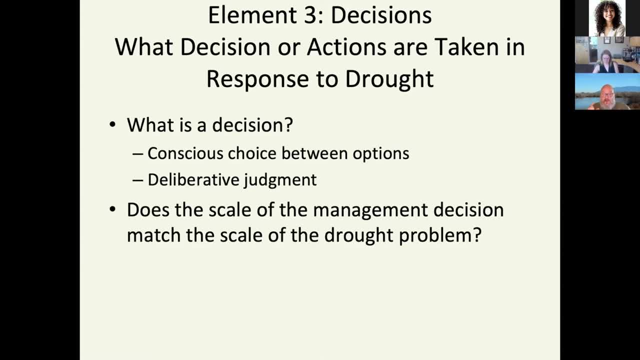 something before, during and after a drought and those who are driving adaptation to droughts. for instance, a dam operator might be critical for the release of water before, during and after a drought, but in some cases- in many cases, not in all cases- they're simply tasked with releasing or not releasing. 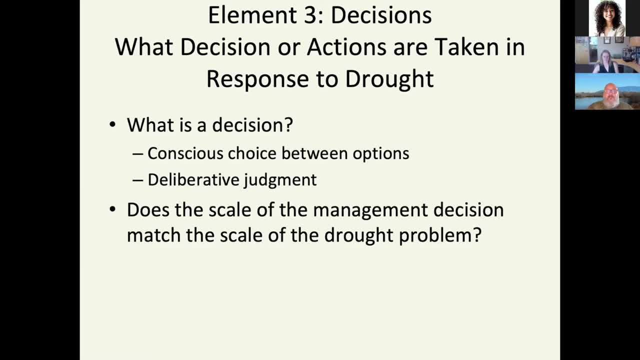 based on decisions that are passed on to them by irrigation districts, federal resource managers, the owners of water, however you want to look at it. second, we also considered whether the scale of the management decision matched the scale of the drought problem. so we needed to be able here to distinguish the 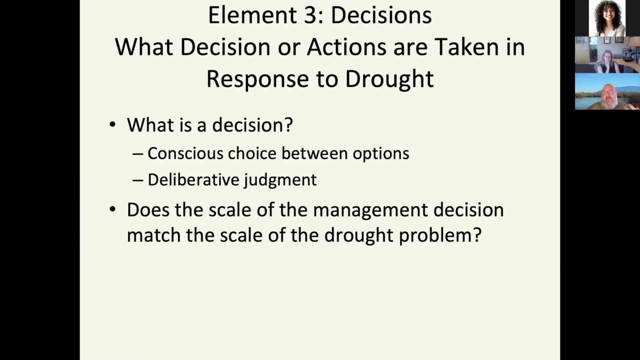 the sort of case of every single individual citizens actions and decisions could be seen as drought management, which we thought was we too difficult to sort of manage that as a drought management typology versus sort of larger scale drought management decisions. again, it's not that the every individual actors decisions don't matter. 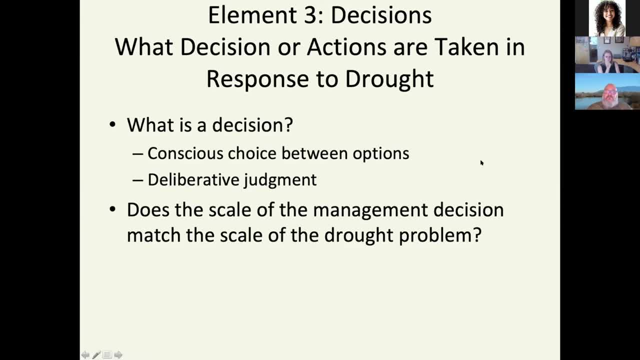 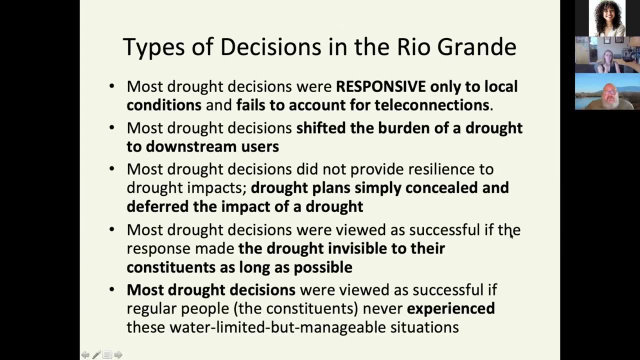 they obviously do, but it's usually it's the scaling of these things in the Rio Grande. I'll just do this very quickly: the types of decisions we ended up sort of identifying, often, as an example of this kind of clustered into a several different categories. most drought decisions we noticed were 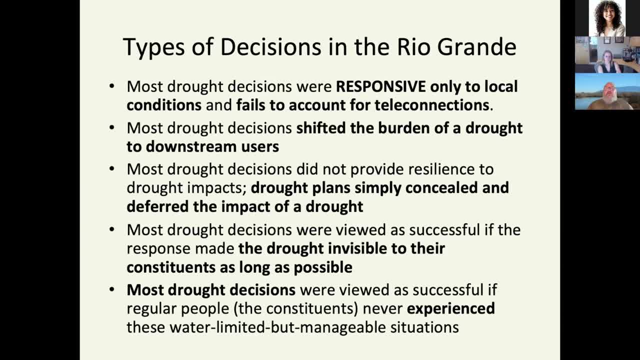 responsive only to local conditions and they failed to account for what are called tele-connections and they failed to account for, often, what was going on way upstream or in other parts of the country, other parts of the world. in sort of making these decisions, most drought decisions shifted the burden of a drought. 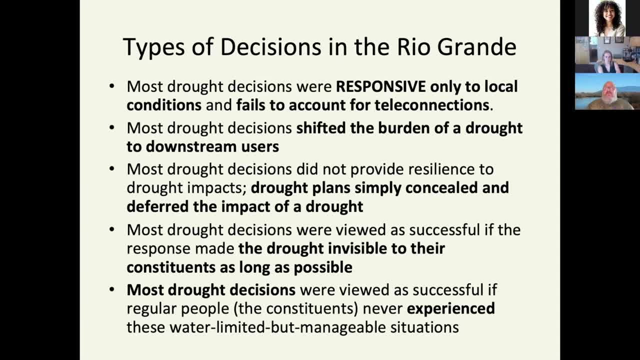 to downstream users. you made a decision based on your own group, your own, your own constituents, and that's what your job was. so that's why they used to be a drought decision, but then they shifted the burden to downstream users of the river. most drought decisions did not provide resilience to drought impacts. 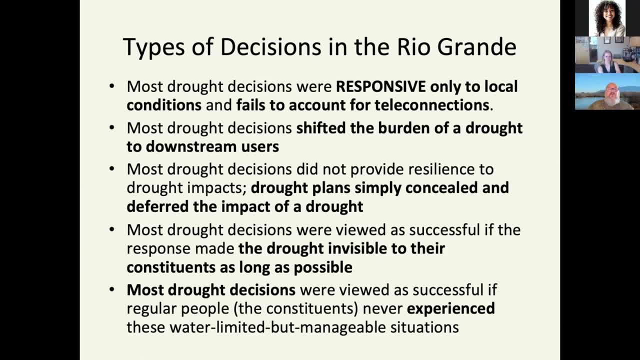 drought plans simply concealed and deferred the impact of a drought. most drought decisions were viewed as successful if the response made the drought invisible to their constituents as long as possible, and that most drought decisions were viewed as successful if regular people- the constituents- never experienced these water limited but manageable situations. again we're. 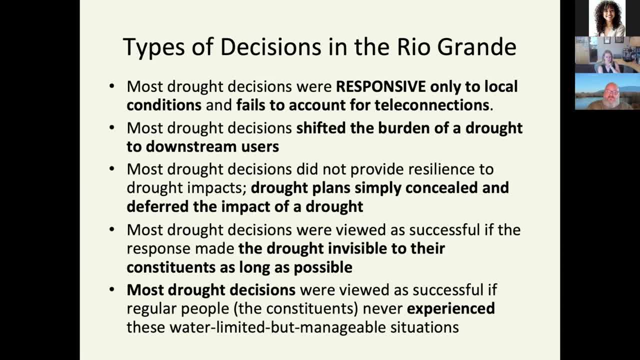 seeing that the kinds of logics that drive a drought decision can inform the typologies of drought decision-making. but you can also then see the implications. if you look a little deeply, scratch at the surface. you can see the implications of why a successful drought decision might actually be very 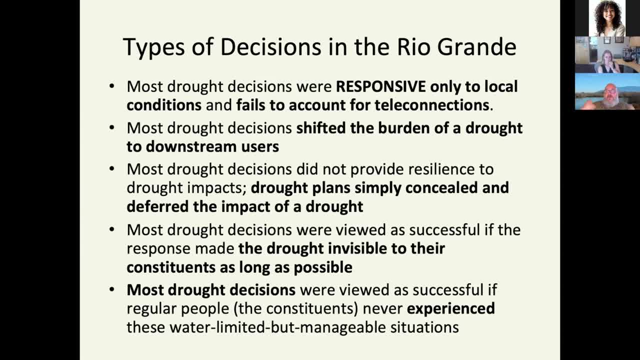 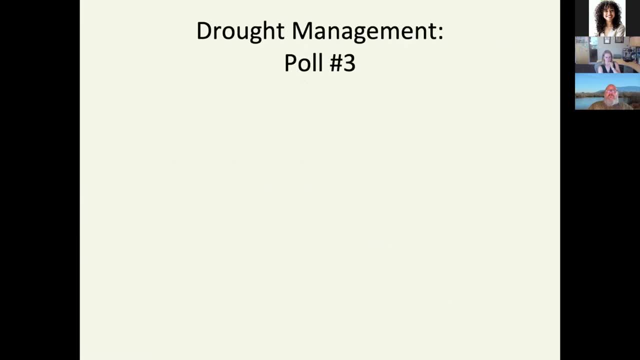 problematic broadly. if the public's never, never, feel drought, then the drought decision was good, but then that might never lead to longer-term changing. so with that in mind, very quickly, let's move on to poll number three, which is very short. it's got a lot of answers, but 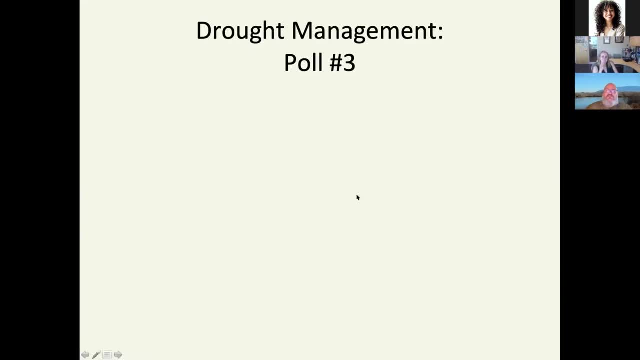 it's actually very short, and one thing I want to stress is that first question is multiple choices, so select all that apply: you, you, you, you, all, you, you, you. okay, I'd like to close this in about 30 seconds. all right, I'm gonna close this now. so, 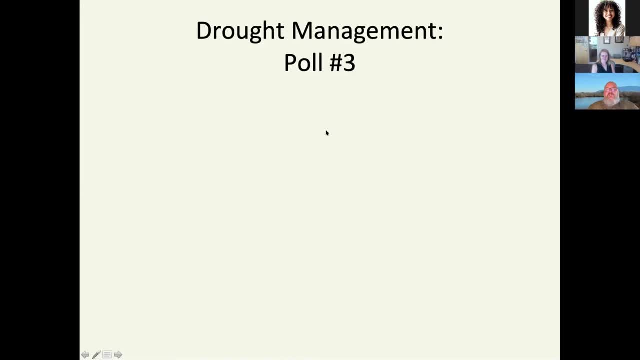 so obviously what I was hoping to see was obviously a lot of people who are being served. I was expecting that, rather than folks who might just say that they're serving one actor or one, one constituency, and- and you clearly see that across here, it's not just that one, for instance, is serving the federal. 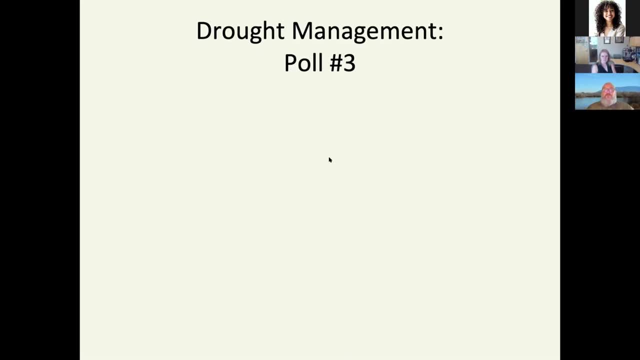 government. almost always you have that narrative somewhere in your job description that when you're serving the federal government you're serving all American citizens, or something like that. but it's this diversity of the people who everybody is serving, I think is critical. you can obviously add all the numbers up. 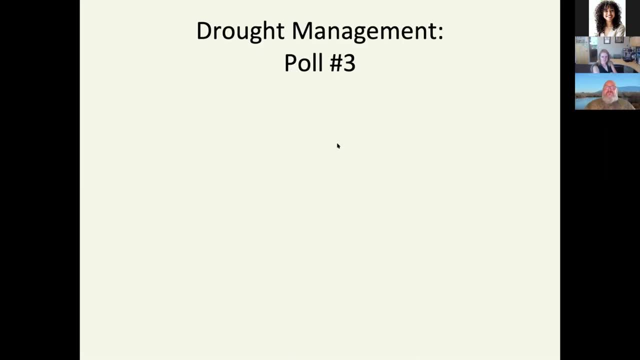 here and it goes well over our 16 participants, the. the issue then ends up being: how is it that you coordinate? and it looks like they're significant. there's there's quite a bit of coordination and active coordination and ways of working with other groups to bring some sort of to bring yourselves together to. 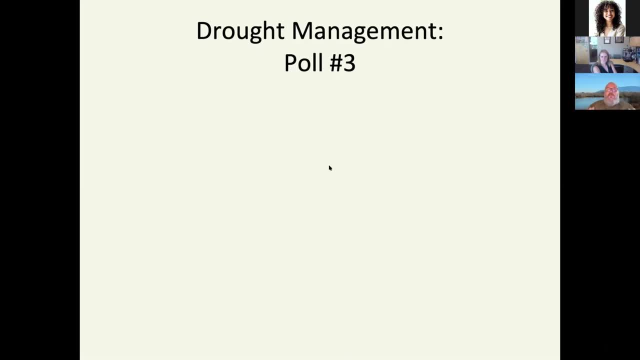 deal with drought problems. but I really was hope, I really wanted to focus on that last question to start with. you know it's sort of it's it. I think it's a real challenging question because often this is the first thing one hears when you start to say, hey, can you make this tough decision from a drought manager? and 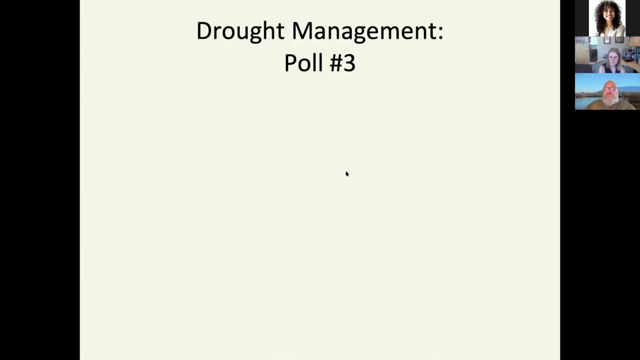 they'll say: well, can't do that because you know the people who I'm serving right now will not allow me to do that, even if it seems get might be good in the long run. so this is hopeful that folks are saying a lot more folks are. 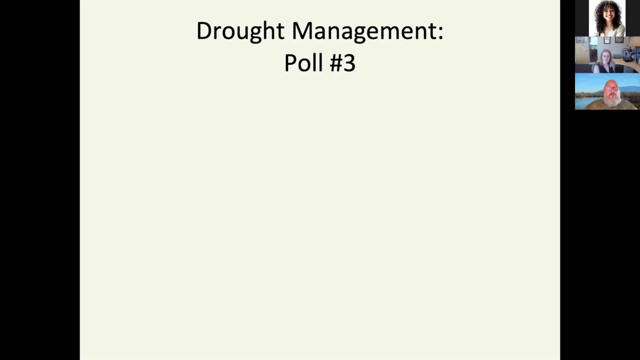 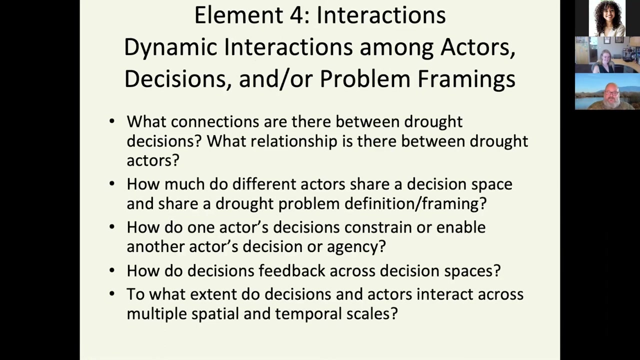 saying yes, and I'm not surprised that we have at least one person saying no, because I that is often the political reality that one faces in practice. Alright, so I have one minute left to get through a couple of slides, but I'll just ignore most of them and just hit. 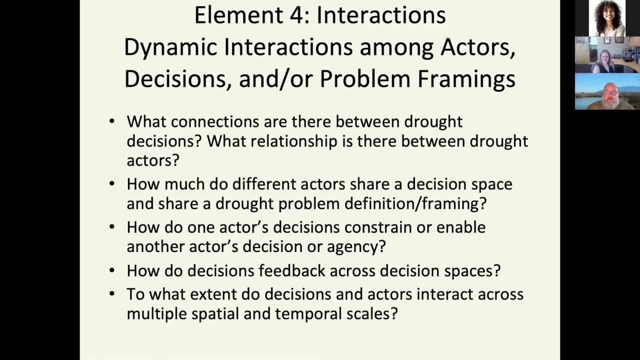 you with the very last element in this, in our typology, So the nature. so obviously this is. these questions were kind of about interactions and the importance of interactions and how they play themselves out, And so we ask a number of questions in deciding how, what, the role of